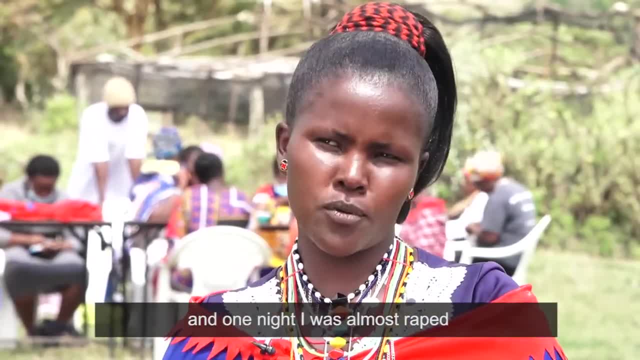 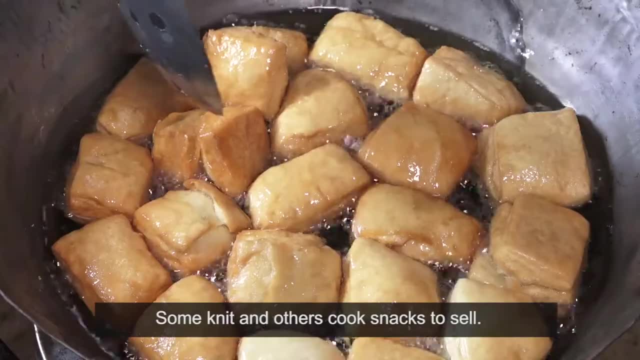 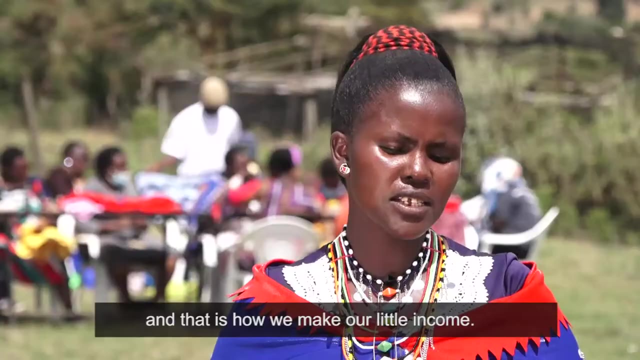 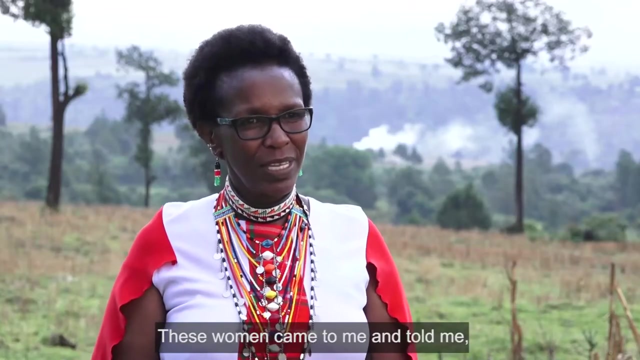 The water tank was closed. but the water tank was closed. Ncamera first, Ncamerafer second, Ncameratır third- Firet fall. The woman came to me. they told me: you are a lady and you are a leader and you will listen. 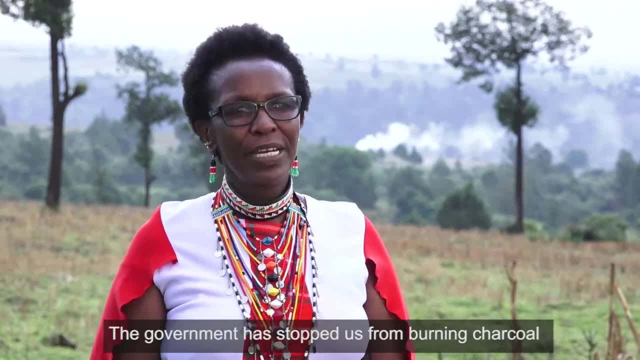 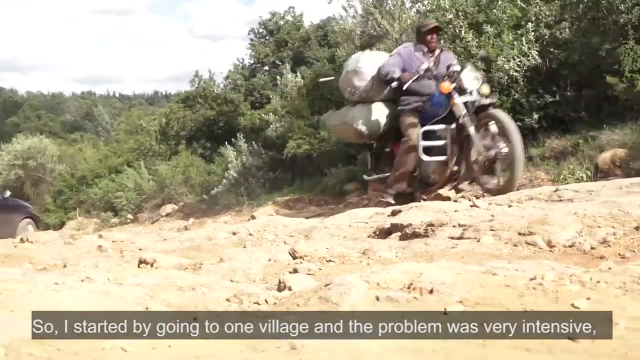 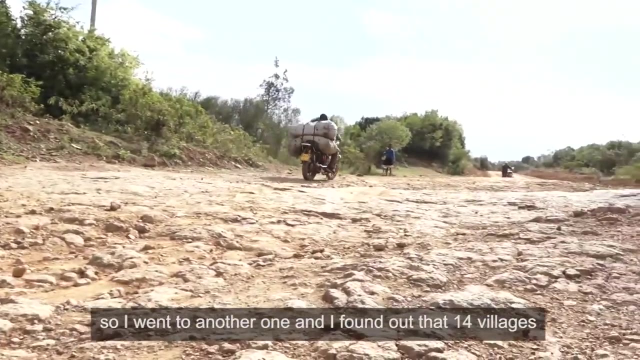 to us. The government has stopped us from banning her charcoal, but they have not given us an alternative. what do we do? so I started going to one village, and then the problem was very intense. I went to another one, and then I found out 14 villages were engaged in charcoal. 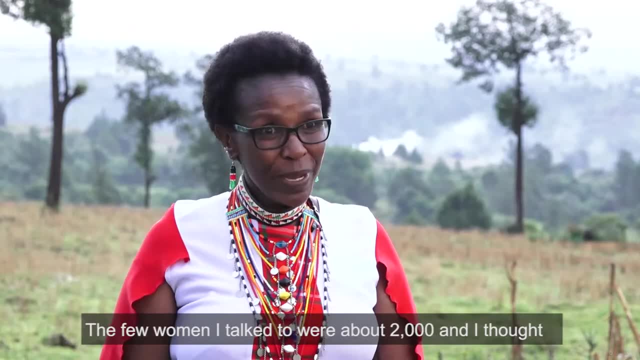 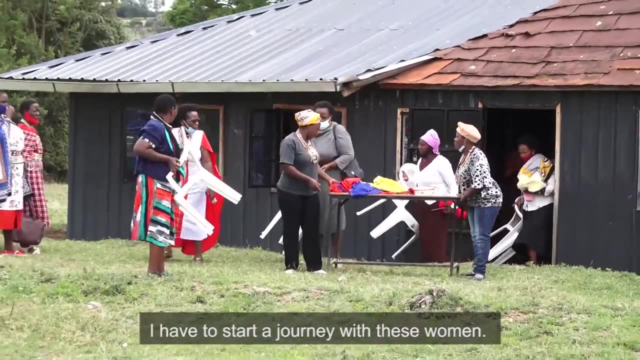 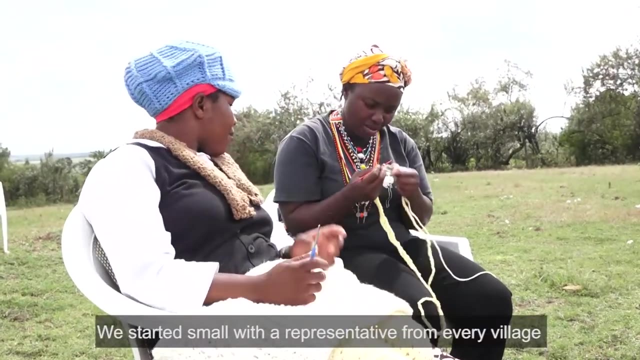 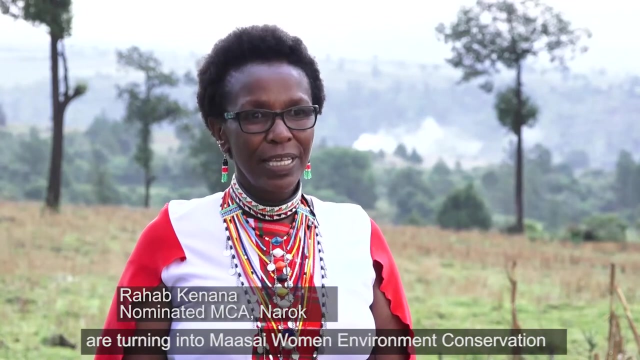 burning and the few women I talked to were about 2,000 and I thought I have to. I have to start a journey with these women. we started small, with a representative from each village. first of all we said we were charcoal producers, but we are turning into Maasai women environment. 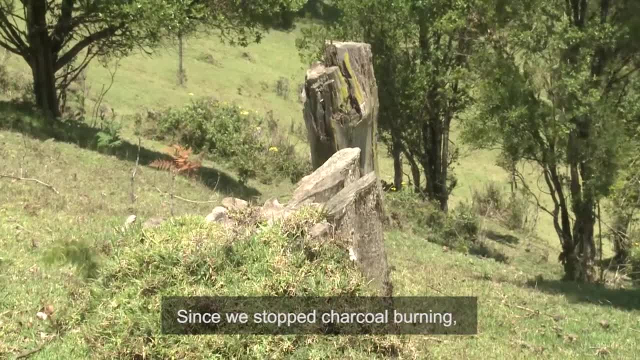 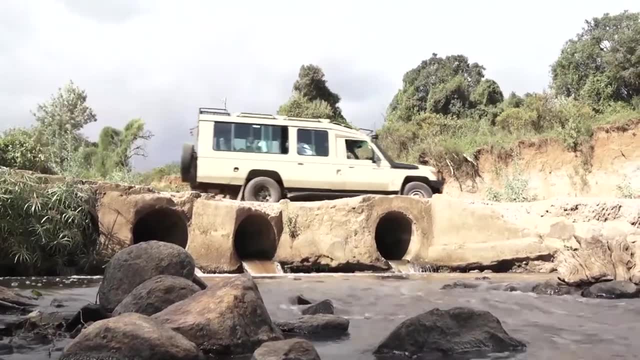 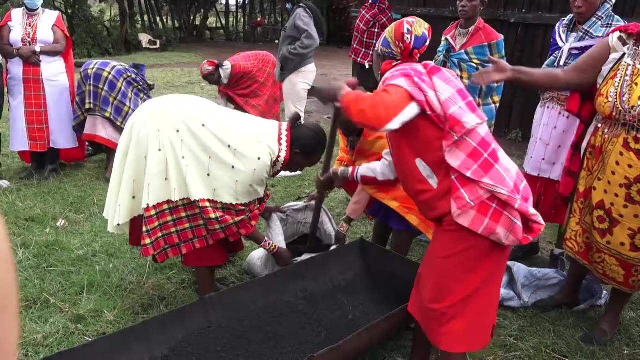 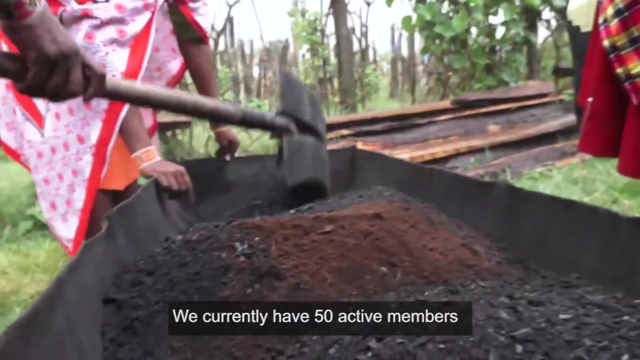 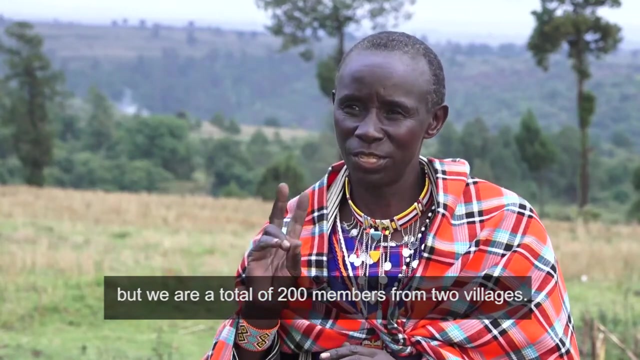 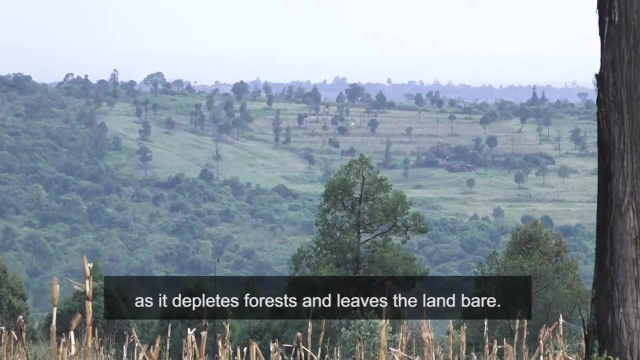 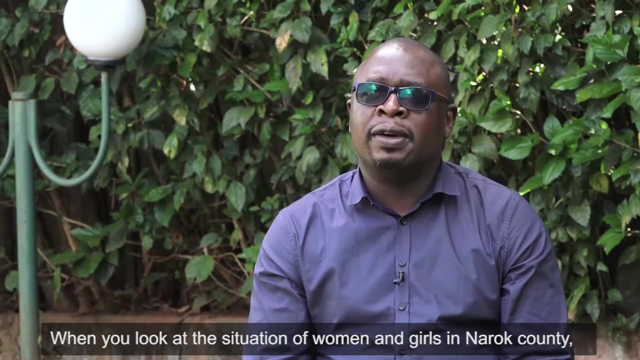 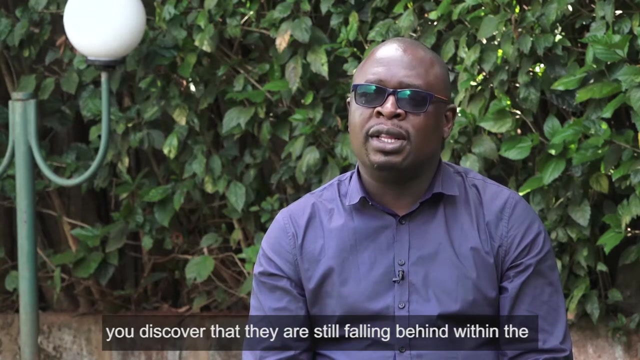 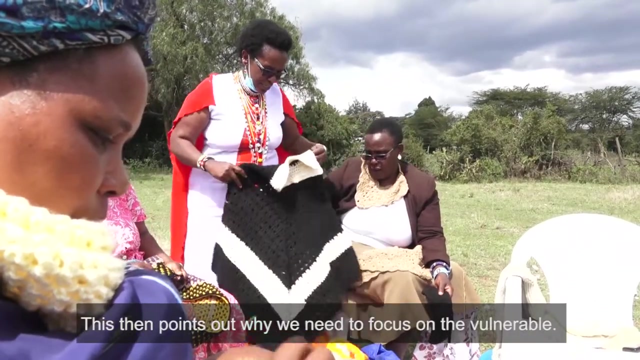 conservation champions. in Narok, just a few kilometers from CIB, another group of vulnerable women is busy making briquettes. when you look at the situation of women and girls in Narok county, you discover that they are still falling behind within the traditional sphere of exclusion, and therefore these points out why we need to focus on the. 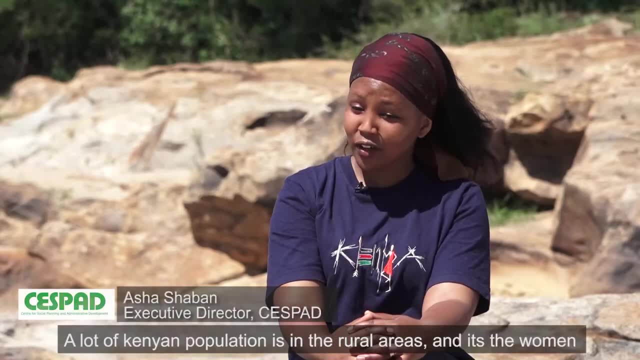 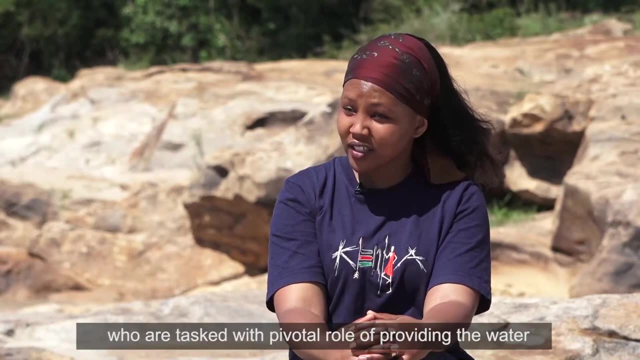 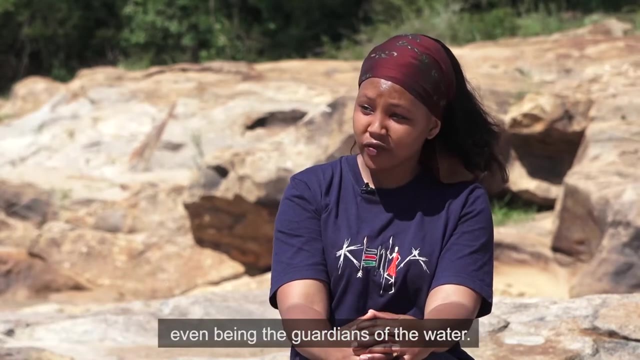 the vulnerable, women play a key role. a lot of a kenyan population is in the rural areas And it's the women who are tasked with that pivotal role of providing the water, of even being the guardians of the water. So they need to sit in the decision-making tables.